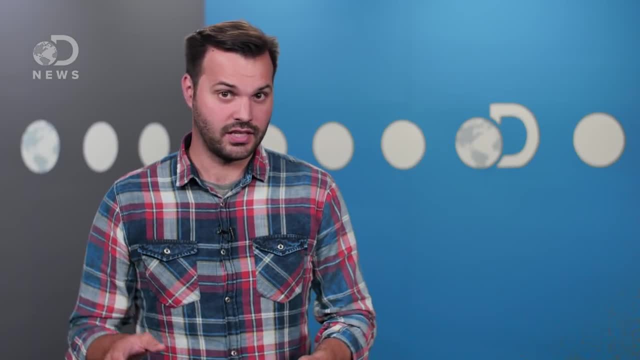 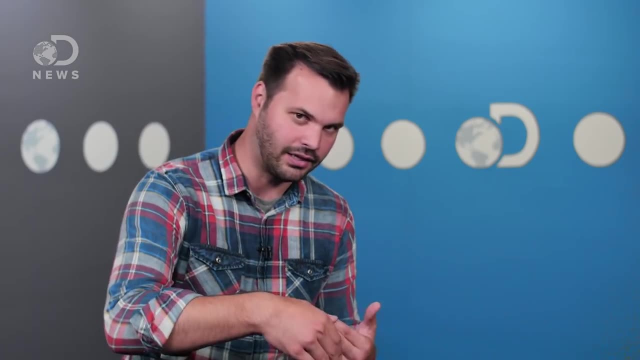 near the center to keep up. This doesn't jive well with the laws of physics. In reality, objects move faster when they're closer to the point they're orbiting around. oh no, otherwise they'd lose the battle with gravity and fall in. 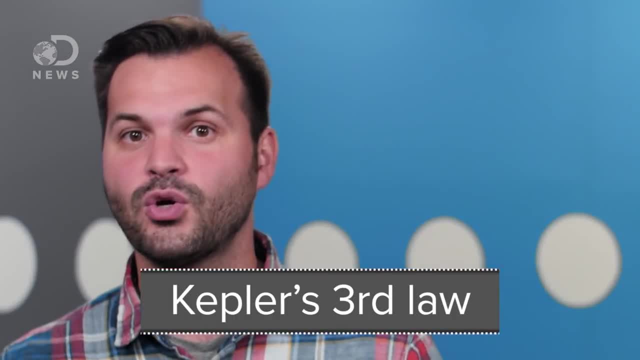 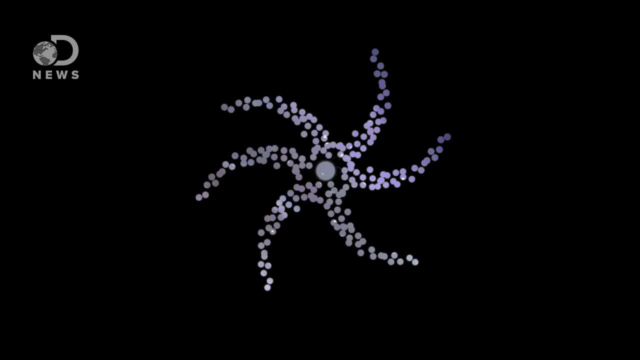 This is Kepler's third law, and it's why Earth's orbit takes a year, while Mercury's is just 88 days. This means, though, that if the arms were made up of the same stars, then, as the galaxy rotates, the arms would get stretched out and wound up like they were. in a giant cosmic taffy machine. Our sun takes around 250 million years to do a lap of the galaxy, Which sounds like a long time, but on an astronomical timescale it's actually pretty quick. At those speeds, spiral galaxies should wind up in the center of the galaxy, and they're. 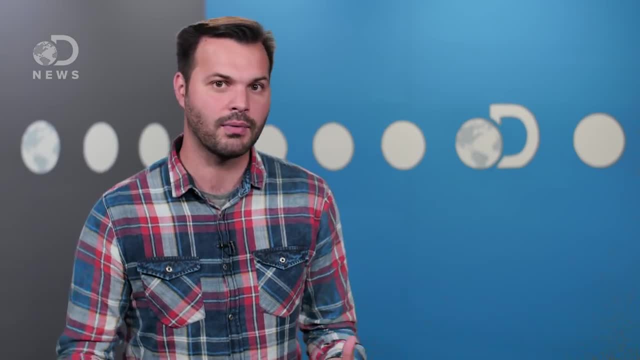 going to be able to move faster than the stars on the tips of the arms. This means that the stars should wind their arms into oblivion before any appreciable length of time, and we shouldn't be observing as many of these galaxies as we do. 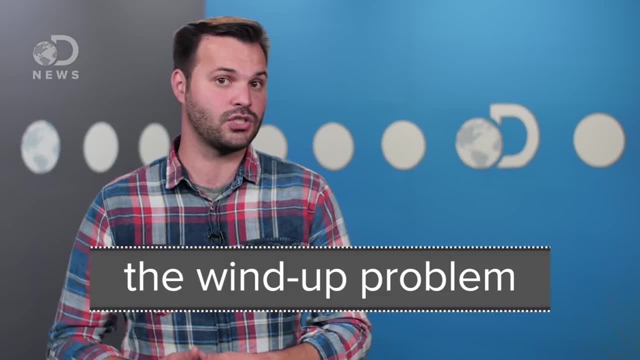 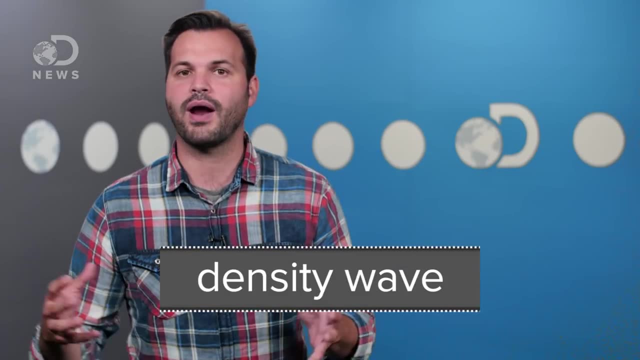 Astronomers call this the wind-up problem, and they've come up with two explanations for the arms. One is that the arms aren't material, but actually the product of a density wave. As stars travel around the galaxy, they'll come to areas where they'll all bunch up, for 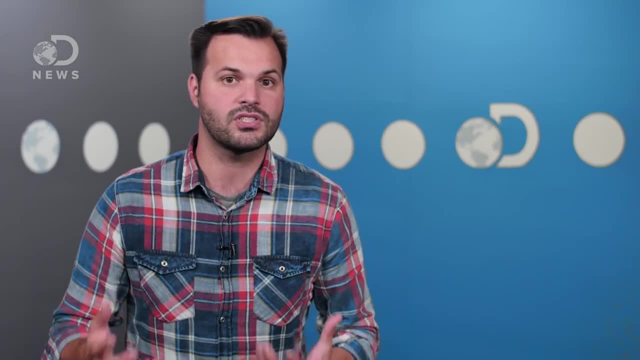 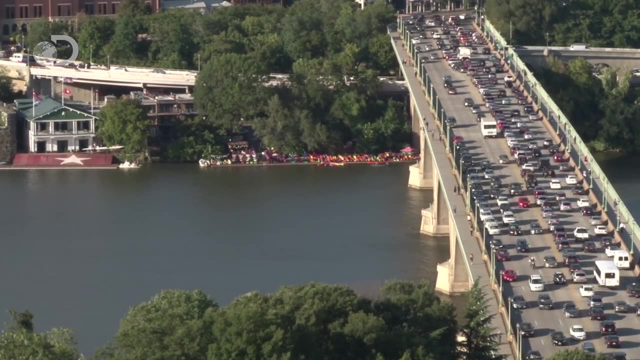 a while and areas where they're more spread out. This means that, though the stars are moving inside of the arms, the arms themselves look pretty stationary. You can think of this like a traffic jam. From afar, the jam appears to stay in one. 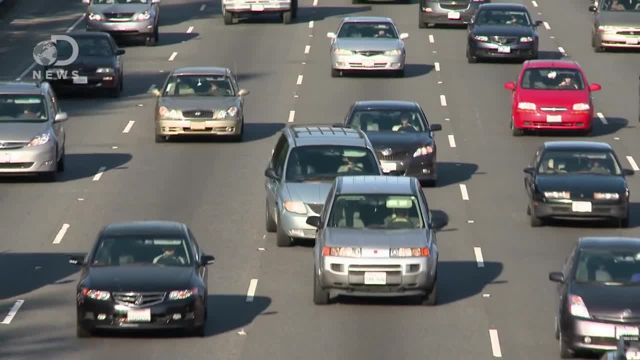 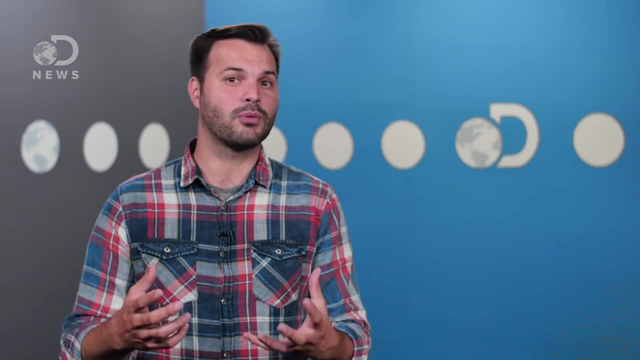 place on the highway, but the cars that make up the jam are actually flowing through it. What would cause these density waves in the first place is still hotly debated. Astronomers have found that spiral arms could be caused by other nearby galaxies or driven by the. 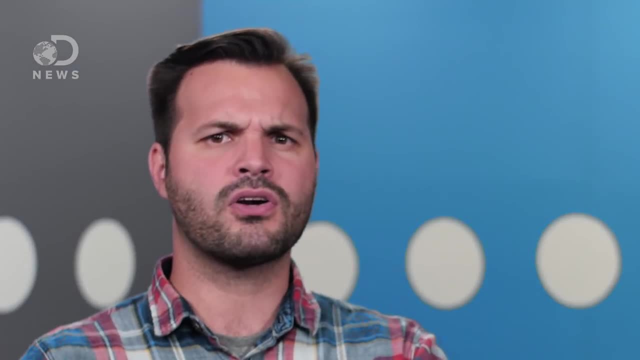 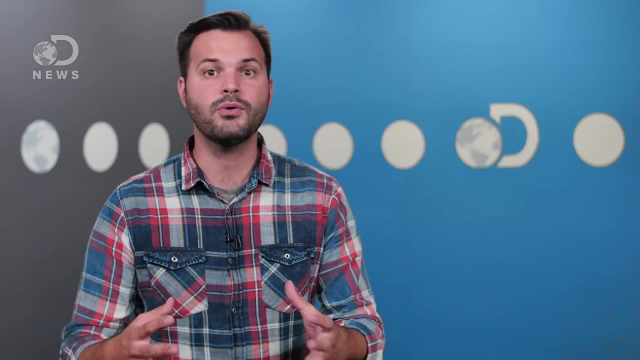 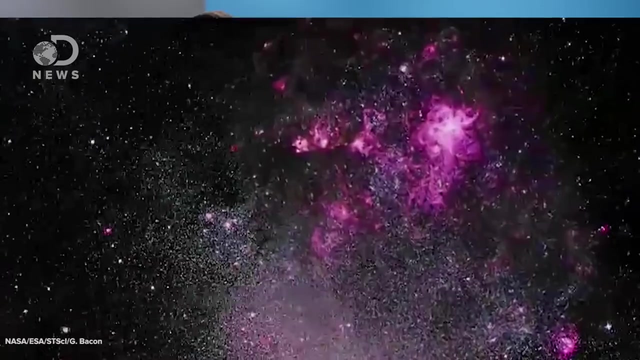 large bar shape at the center of some galaxies, But these bars and companion galaxies are not universal, so explaining galaxies that have neither with the density wave model is tricky. The other popular explanation is stochastic, self-propagating star formation, but its friends call it SSPSF. The basic idea behind it is star formation in a galaxy causes a shock. 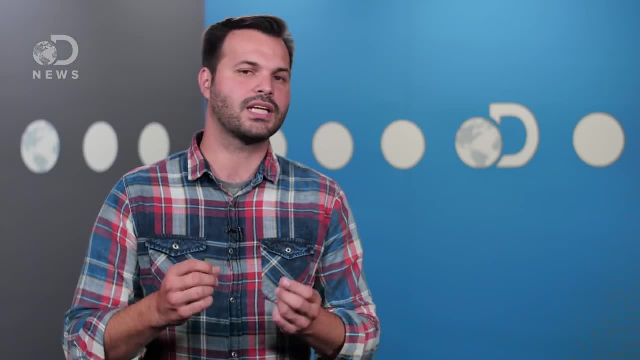 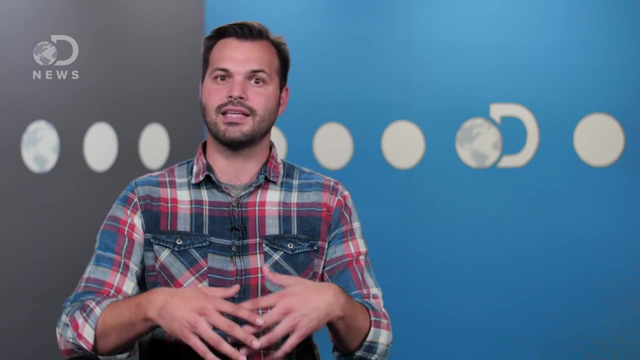 wave that kicks off more star formation. The rotation of the galaxy stretches the bright new stars into familiar spiral arms and they burn out and die as the chain reaction propagates and the arms move on. It's possible SSPSF and the density wave model actually work together. 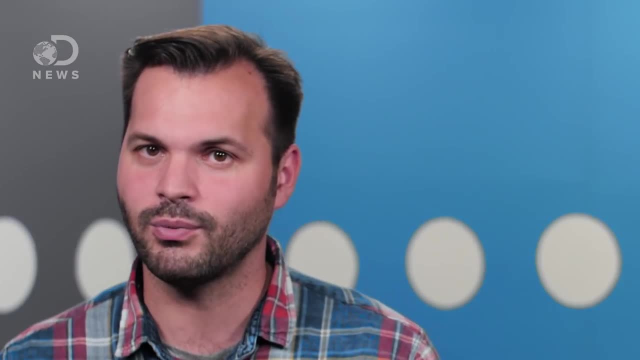 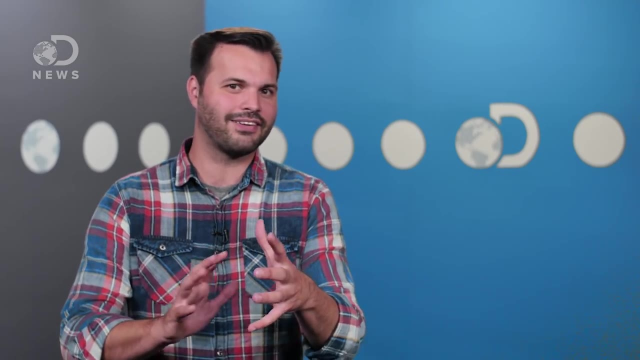 and stars are formed in the denser areas, making the arms look brighter with their hot new stars. So those are the most accepted explanations of spiral formation, but some of the finer points, like figuring out if these spirals are long-lived or transient features, can.